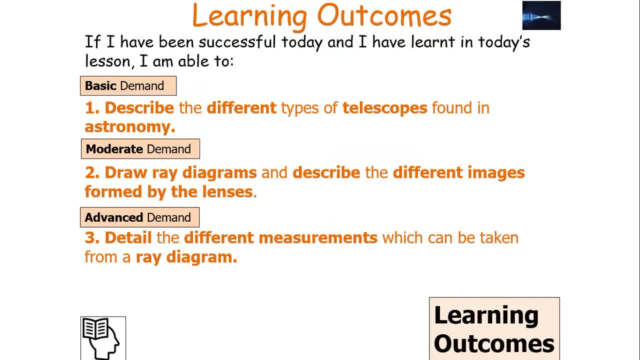 telescopes. So if you are successful and you've learned in today's lesson, you should be able to describe the different types of telescopes found in astronomy, draw ray diagrams and describe the images formed by the lenses, and then detail the different measurements which can be taken from a 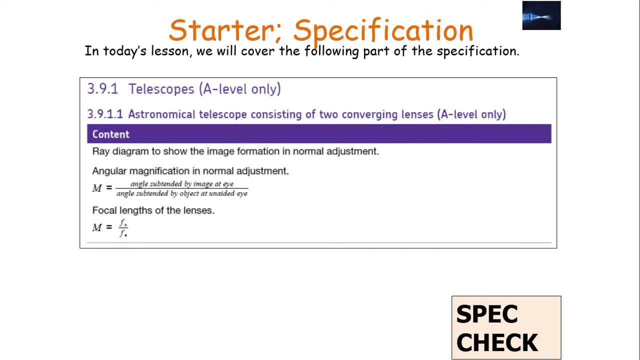 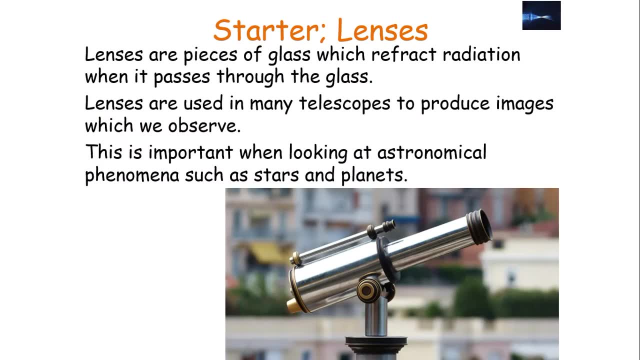 ray diagram, which falls into the following part of the AQA A-level physics specification, which is part of the astrophysics option. So lenses are pieces of glass which refract radiation when it passes through the glass, and lenses are used in many telescopes to produce images which we observe. 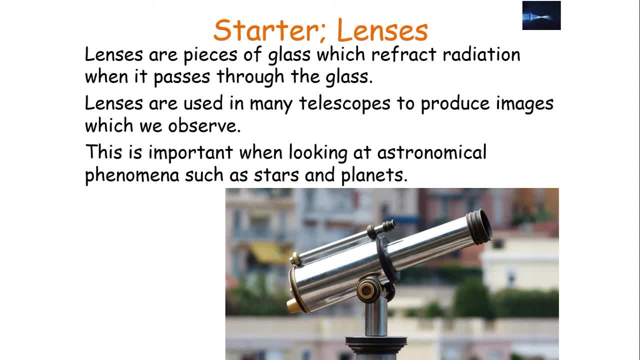 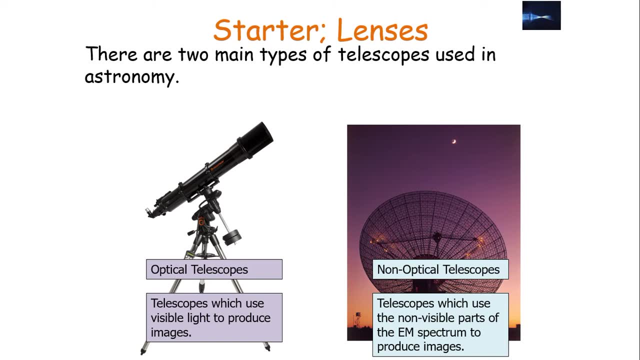 which is important when we look at astronomical phenomena such as stars and planets. So basically, lenses change the direction of electromagnetic radiation via the process of refraction. Now there are two main types of telescopes used in astronomy. We've got optical telescopes, which are telescopes which use visible. 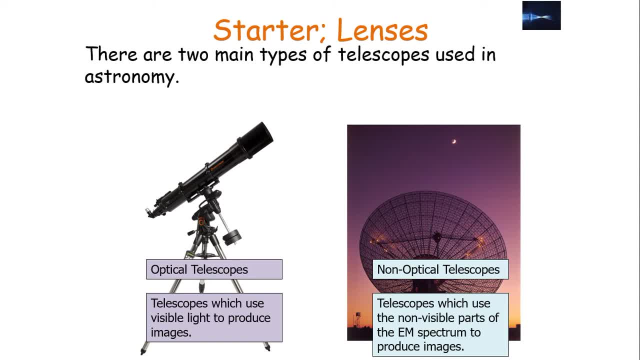 light to produce images, and non-optical telescopes, telescopes which use the non-visible parts of the electromagnetic spectrum to produce images. So the optical telescopes are the telescopes more familiar to the public, but non-optical telescopes are the more commonly. 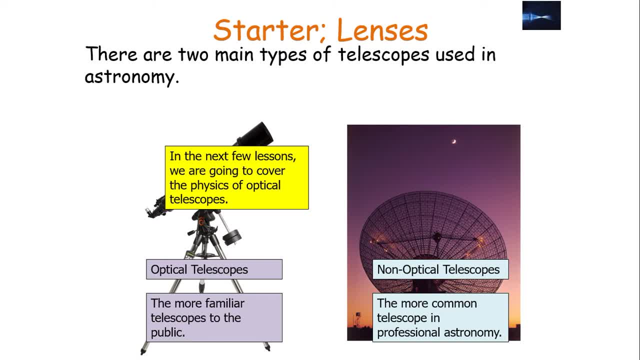 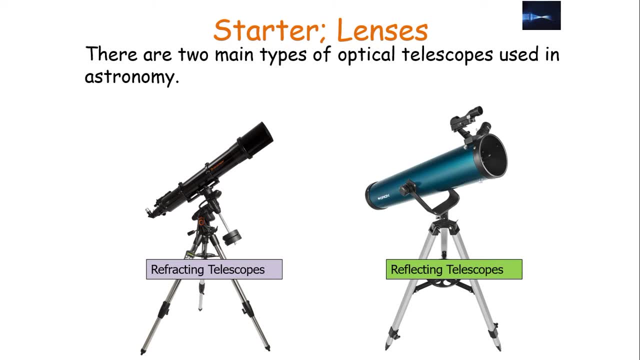 used telescopes in professional astronomy. So in the next couple of lessons we're going to cover the physics of optical telescopes before moving on to non-optical telescopes. So there are two main types of optical telescopes used in astronomy: refracting telescopes and reflecting telescopes. 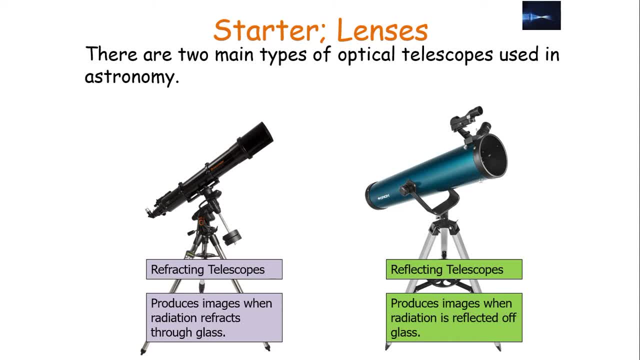 So refracting telescopes produce images when radiation refracts through the glass, whilst in reflecting telescopes they produce images when radiation is reflected off the glass. So refracting telescopes are expensive, they're easily distorted and are difficult to manufacture, whilst reflecting telescopes tend to be cheaper. 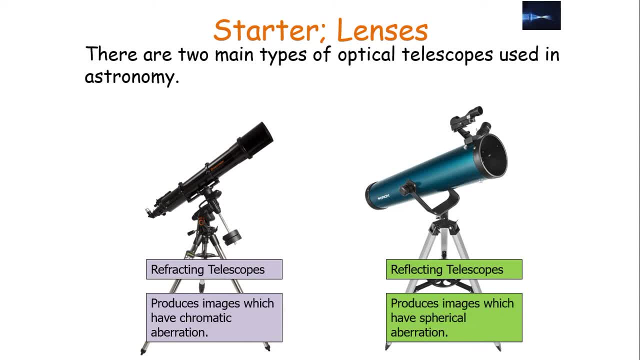 can be supported more easily and are easier to manufacture, Whilst refracting telescopes produce images which have a chromatic aberration, whilst reflecting telescopes produce images which have a spherical aberration. Now, a refracting telescope tends to consist of two converging 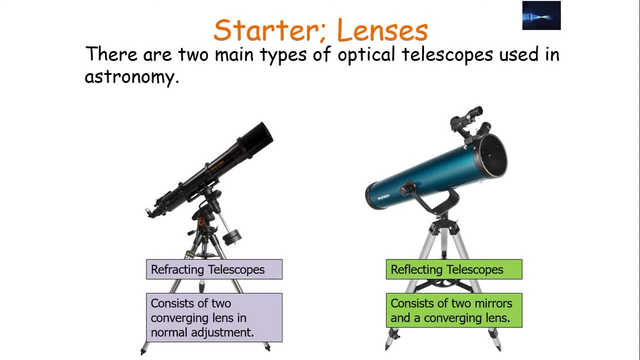 lenses in what we call normal adjustment and reflecting telescopes consist of two mirrors and a converging lens. Now we actually call that arrangement the Cassie-Grain arrangement. Now, in today's lesson we're going to focus on the physics behind refracting telescopes. 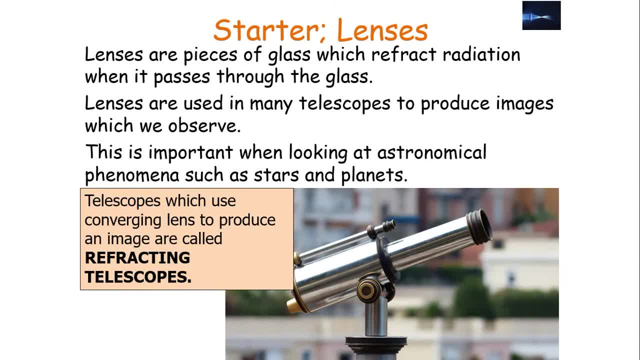 which builds on the concepts you've covered in GCSE Physics. So, as we mentioned before, telescopes which use converging lenses to produce an image are called refracting telescopes. So to understand how refracting telescopes work, we must understand the physics of the converging lens. 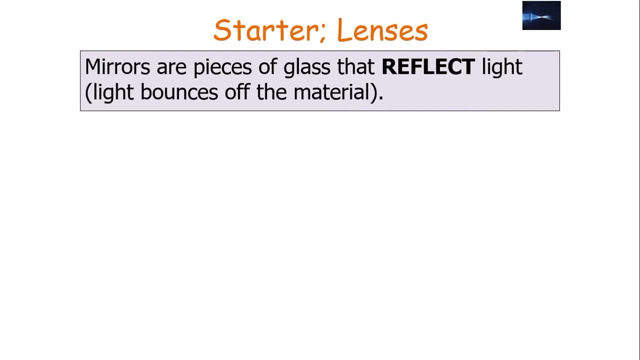 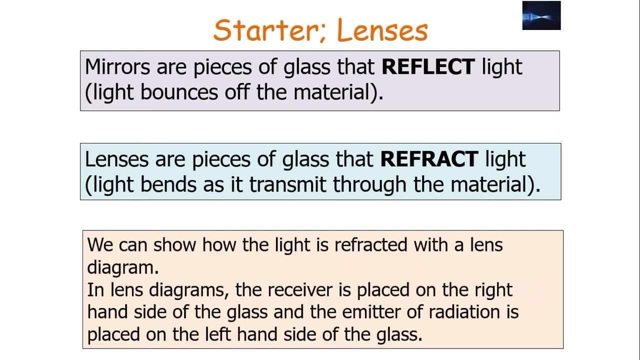 Now, mirrors are pieces of glass that reflect light, so the light bounces off the material, whilst lenses are pieces of glass that refract light when light bends as it transmits through the material. Now we can show how light, or any radiation, is refracted with a 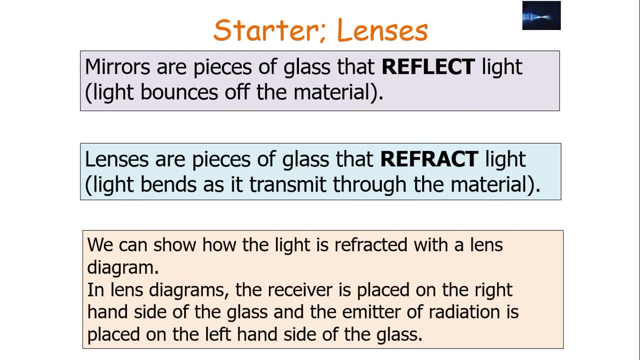 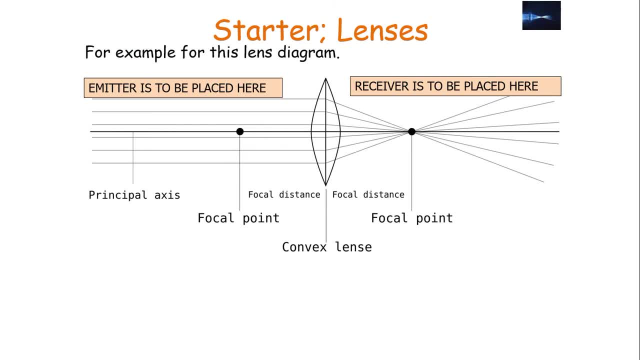 lens diagram. Now, in a lens diagram, the receiver is placed on the right-hand side of the glass and the emitter of the radiation is placed on the left-hand side of the glass. So this shows our lens diagram, with the emitter on the left-hand side and the receiver on the right-hand side. 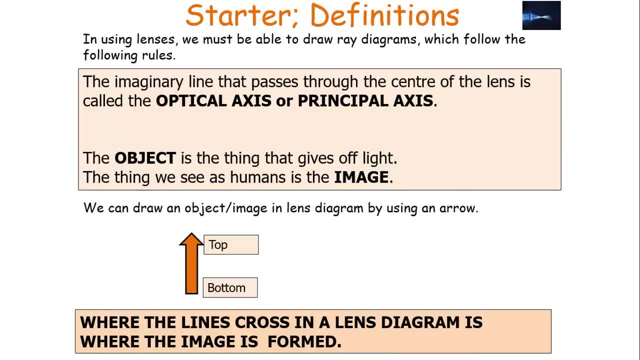 Now to draw accurate lens diagrams. we've got to follow some fundamental rules Now in using lenses. when we draw ray diagrams we use the following rules: The imaginary line that passes through the centre of a lens is called the optical axis, or the 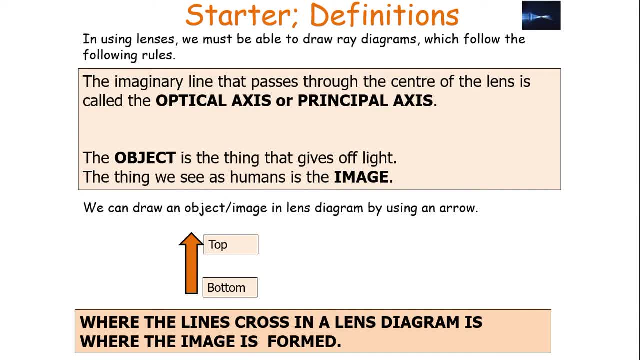 principal axis. The object is the thing which gives off light or radiation. The thing we see as humans is the image. Now we can draw an object or image in a lens diagram by using an arrow, with an arrowhead representing the top of an object and the bottom of an arrow representing the bottom of 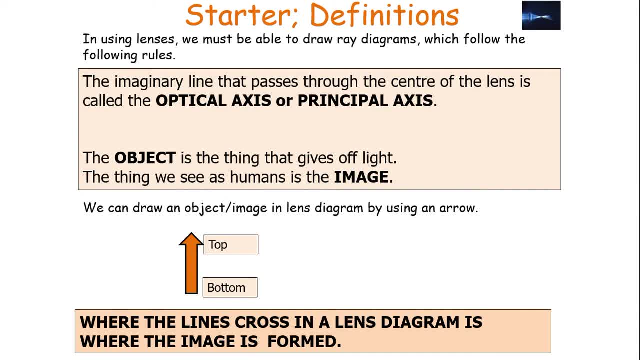 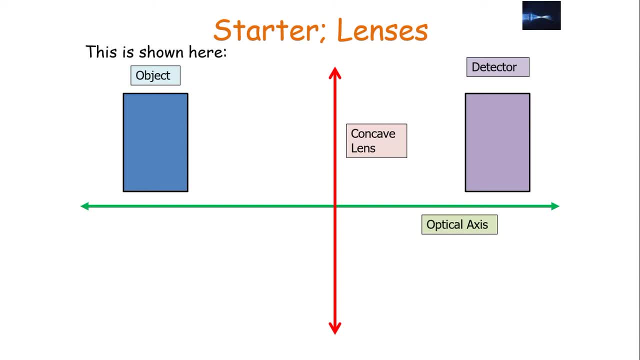 an object. Now, where lines cross, we can draw an image of an object. Now we can draw an image of an object across in a lens diagram. an image is formed So we can show this example in this particular picture or in this particular drawing here of a ray diagram. Now, there are two types of 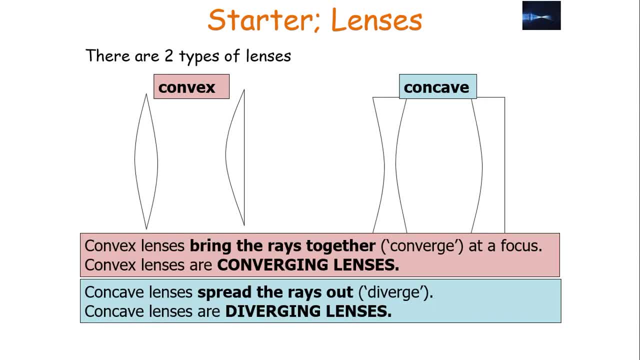 lenses: convex lenses and concave lenses. Now, convex lenses bring the rays together or converge the rays at a focus, So convex lenses are called converging lenses, whilst concave lenses spread the rays out or diverge the rays. So we call those types of lenses convex lenses. Now we can. 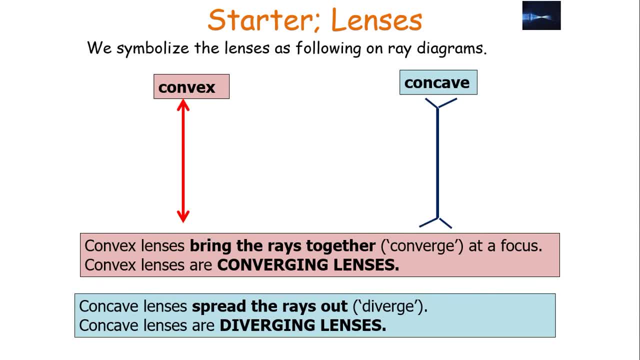 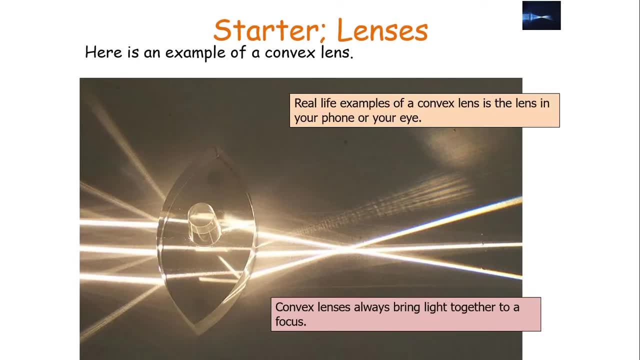 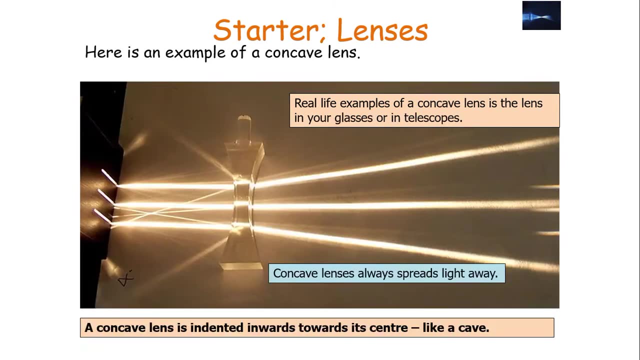 symbolise the lenses with the following images on ray diagrams. So here's an example of a convex lens. Now, a real life example of a convex lens is the lens in your phone or your eye. Now, convex lenses always bring light together to a focus. Now here's what a concave or diverging lens looks. 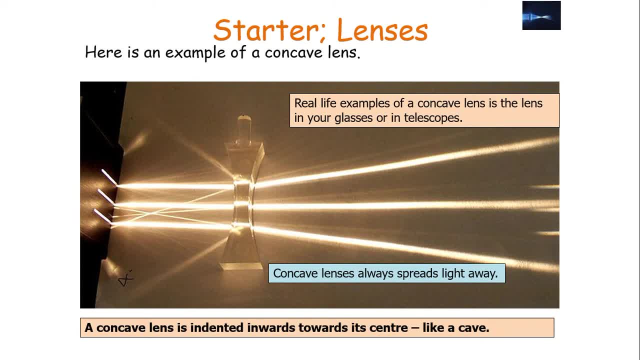 like. and again, these are used sometimes in telescopes and sometimes in glasses. Now, concave lenses always spread light away. Now, a concave lens is a lens that is used to see the rays of a. a concave lens is indented inwards towards the center, like a cave, given its name. Now, in practice, 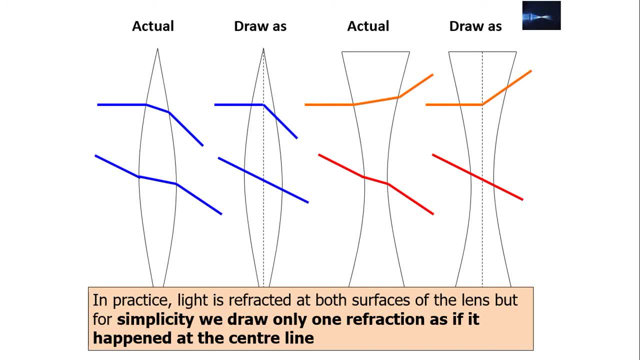 light or any type of radiation is refracted at both surfaces of the lens, where the radiation enters the lens and when it leaves the lens. but for simplicity's sake we only draw one effective refraction, as if it happened at the center of the lens. but in actuality it happens when the 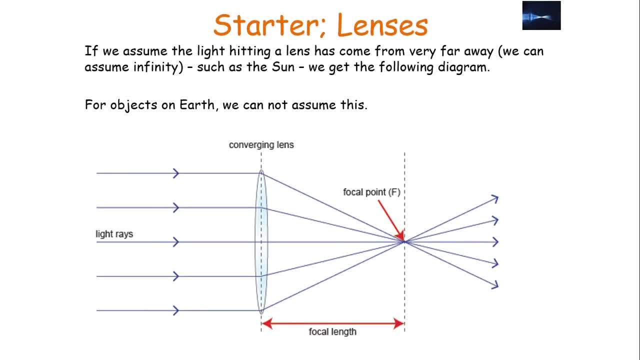 radiation enters the lens and when it leaves the lens. Now, if we assume the light or any radiation hitting the lens has come from very, very far away, or infinity, such as a star like the sun, we get the following diagram: Now for objects on earth. we tend not to assume this Now, as the light has traveled. 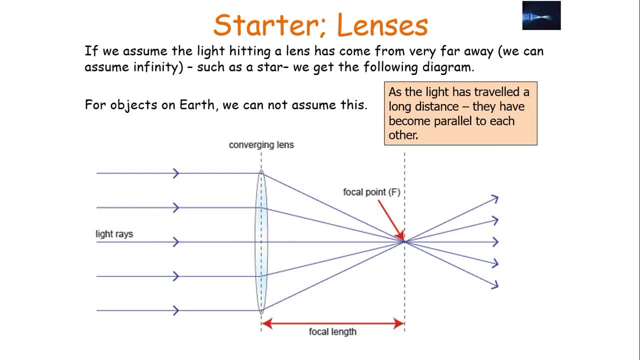 a long distance from the star. we say that the light rays have become parallel to each other and with the optical axis. So, as a result, when this happens with convex lenses, it makes the rays converge to one point, which we call the principal focus or the focal point, Now the perpendicular 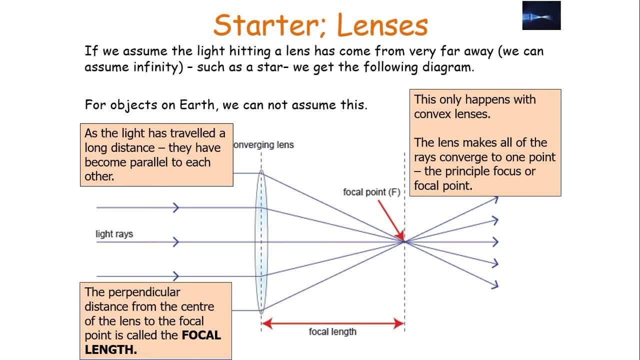 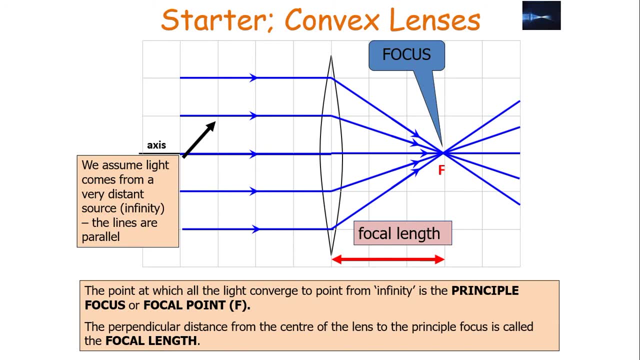 distance from the center of the lens to the focal point is called the focal length. So let's just clarify what we've learned. When light has traveled from infinity a very distant source, such as a star or a planet, the lines are parallel to each other, and with the optical axis, The point at which all the 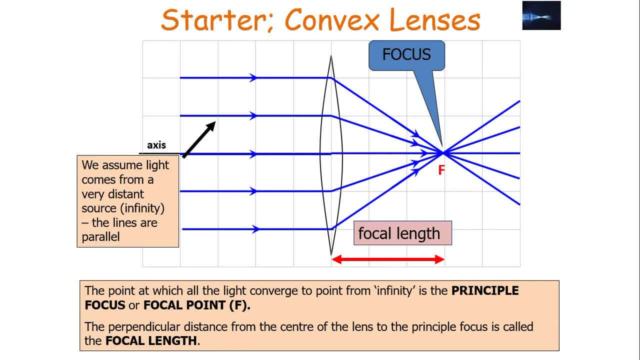 light converge to a point from infinity is called the principal focus or focal point. The perpendicular distance from the center of the lens to the principal focus is called the focal length. Now, rays which have traveled a great distance from the center of the lens to the focal point are called the focal point. 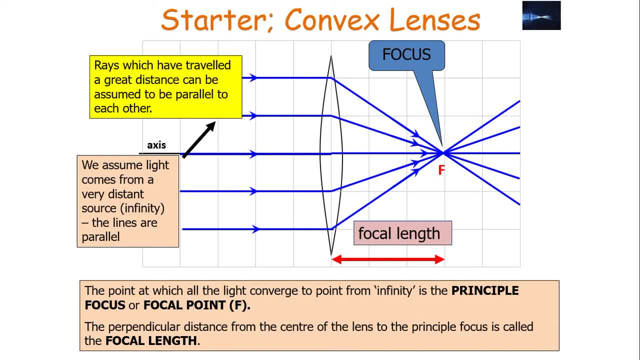 When the optical axis is parallel to the distance from the center of the lens to the focal point. the distance can always be assumed to be parallel to each other and the optical axis. So rays from any astronomical object can be considered this because they've traveled a great distance. Now, rays which 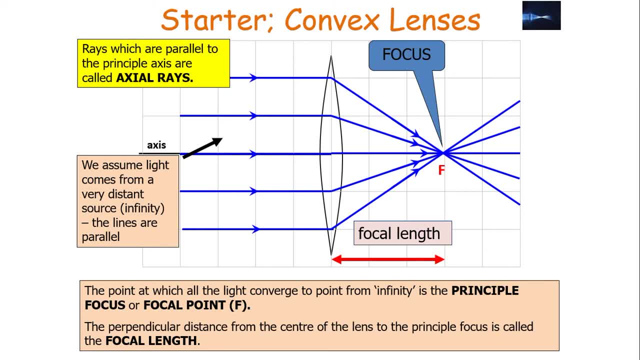 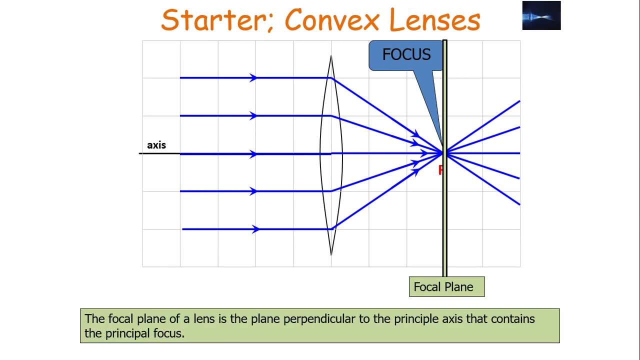 are parallel to the principal axis, or the optical axis, are called axial rays. This is because the rays, like we said before, are parallel to the axis. So all axial rays converge at the principal focus after they pass through a convex lens. So the focal plane of a lens is called the focal length and the 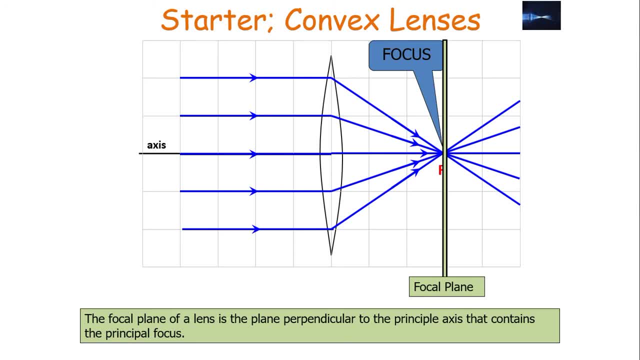 lens is the plane perpendicular to the principal axis that contains the principal focus, as shown in this particular diagram. Now, like we mentioned before, the focal length of a lens can also be defined as the perpendicular distance from the centre of the lens to the focal plane itself. 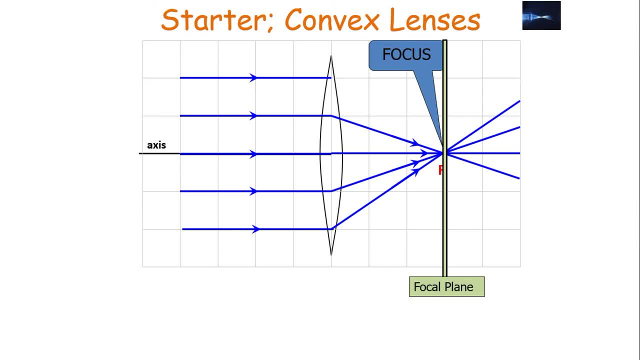 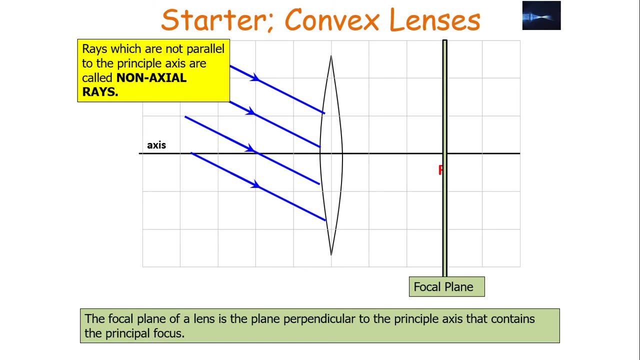 So here we've got the focal plane of this particular lens, because it's a plane of a 2D surface which is perpendicular to the optical or principal axis and contains the focal point or focus of the lens. Now, rays which are not parallel to the principal axis are called. 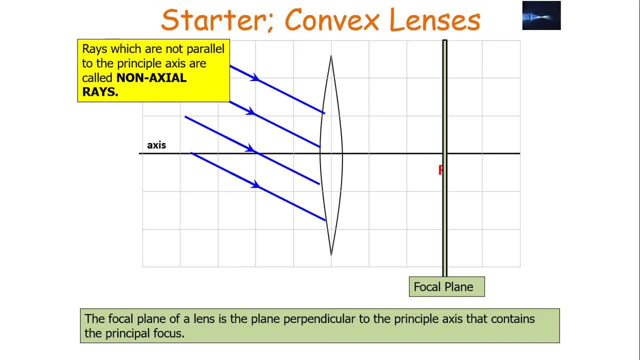 non-axial rays. Now you'll notice they are parallel with each other, but they're not parallel with the principal axis. So non-axial rays, as I said before, can still be parallel to each other because they've travelled a great distance. Now rays hitting the lens are much more likely to be. 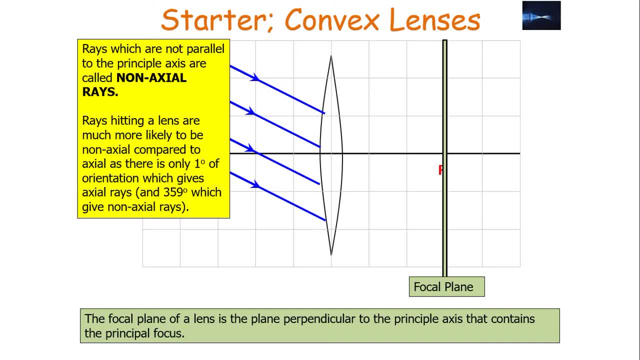 non-axial Compared to axial, as only one degree of orientation gives axial rays, whilst the other 359 degrees give non-axial rays. Now non-axial rays converge and form an image somewhere on the focal plane, but not at the focal point. Now the position of the image can be determined by the non-axial ray. 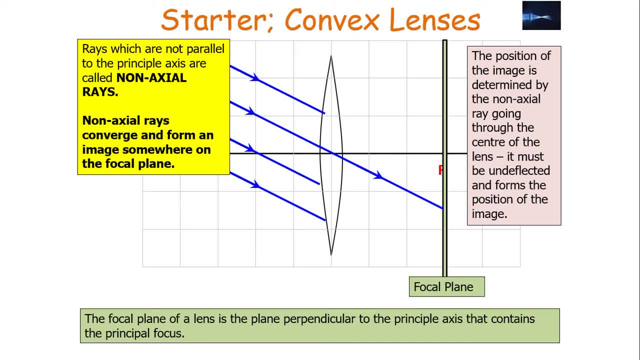 going through the centre of the lens because, as we'll talk about in a bit, one rule of lenses is that if a, if a ray of radiation travels through the centre of a lens, it must be undeflected. So the non-axial ray, 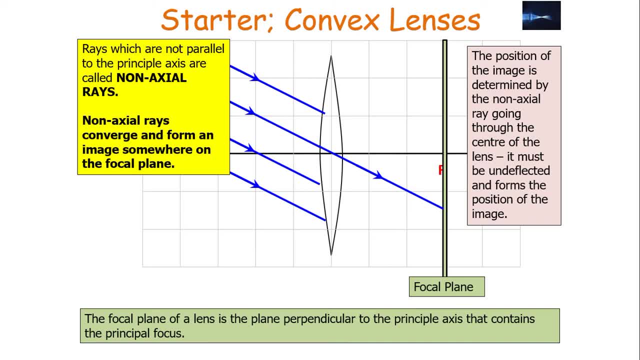 which travels through the centre of the lens, is undeflected and therefore will travel straight through, as it's shown on the particular diagram, And because, as we know, the image has to be produced on the focal plane, at that point we know that that's where the image must be. 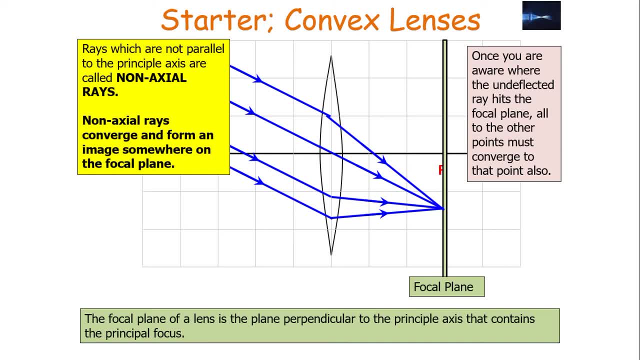 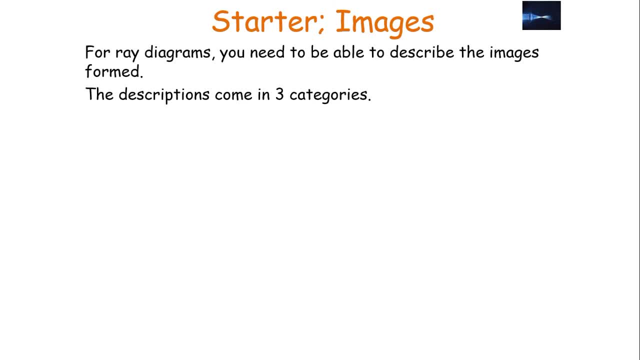 Because once you are aware that where the undeflected ray hits the focal plane, all the other points must converge to that point as well. Now for ray diagrams, you need to be able to describe the images formed, and the images come in three categories. Category one: if it's upright. 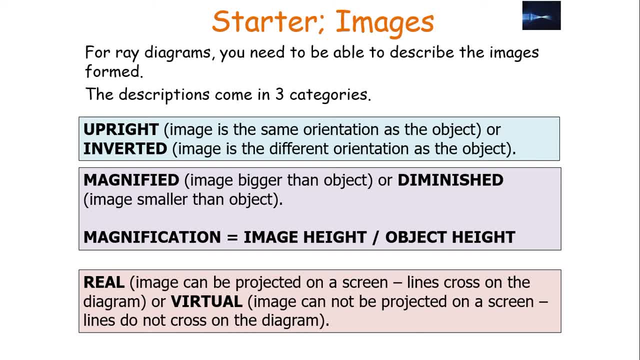 which is the image, is the same orientation as the object or inverted- the image is different. is a different orientation as the object. The object can be either magnified when the image is bigger than the object, or it can be diminished. the image is smaller than the object. 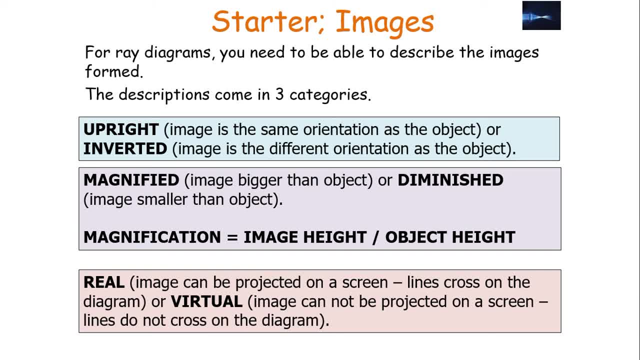 And magnification can be worked out with the equation image height divided by object height. And finally, you can describe your image as either a real image, where the image can be projected on a screen- the lines actually cross in the diagram- or virtual. 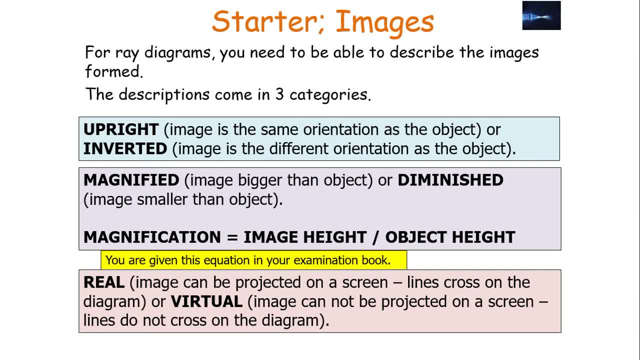 the image cannot be projected on a screen. the lines do not cross on a diagram. Now you are given the magnification equation in your examination books. You don't need to memorise that particular equation for your examination Now. magnification has no units, it's just a ratio. Now a magnification. 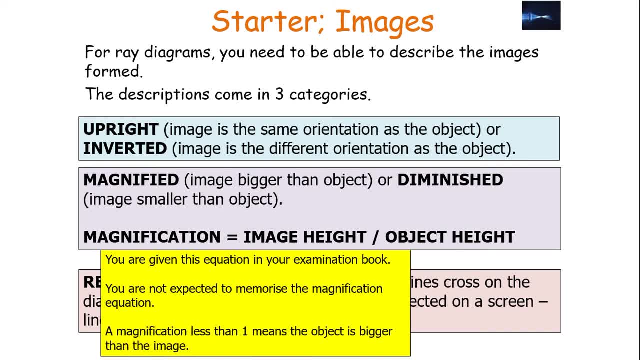 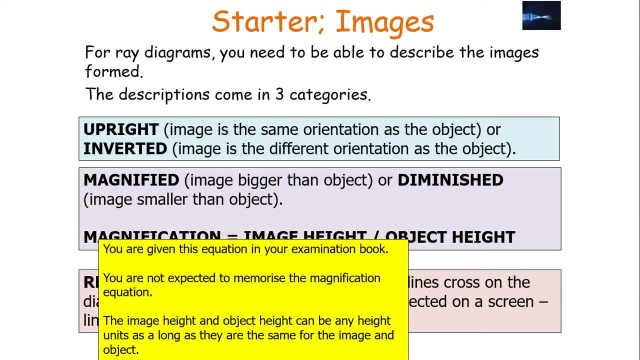 greater than 1 means the image is bigger than the object. a magnification less than 1 means the object is bigger than the image. Now, the image height and object height can be in any height units- millimetres, centimetres, metres- as long as they're the same for the image in the object. 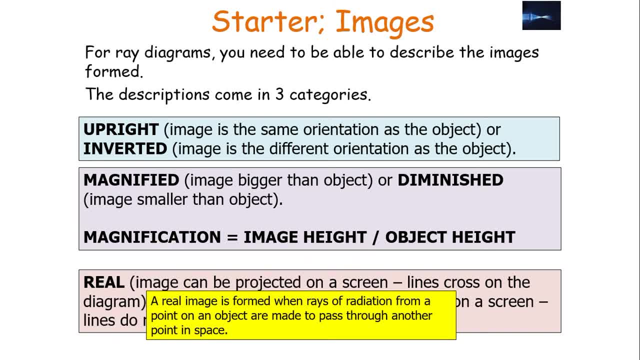 Now a real image is formed when the rays of radiation from a point on an object are made to pass through another point in space. So the light rays are actually there and the image can be captured on a screen. A virtual image is formed when light rays from 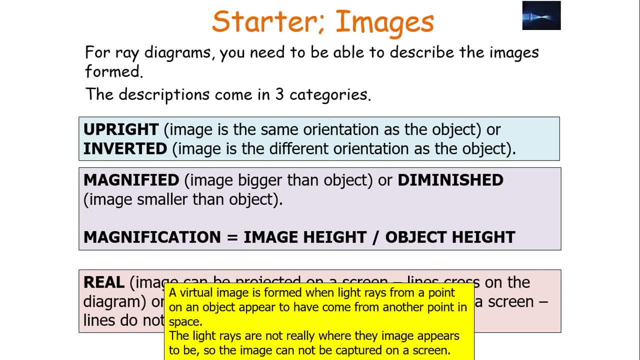 a point on an image appear to have come from another point in space, So the light rays are not really where the image appears to be, so the image cannot be captured on a screen. A convergent lens can form both real and virtual images, depending on where the object is. If the object 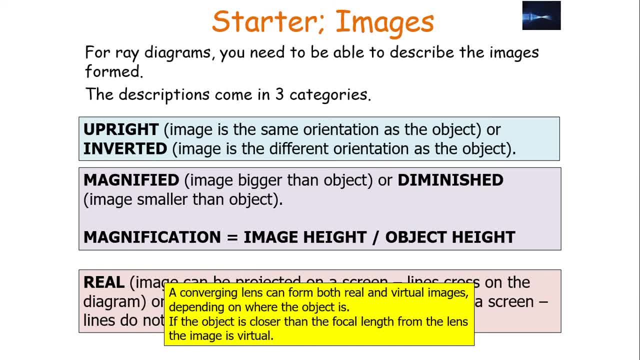 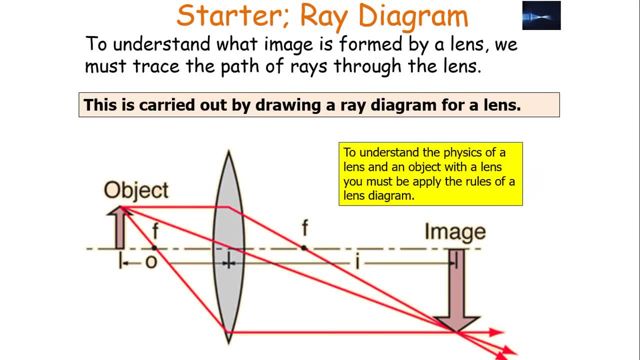 is further than the focal length away from the image. it's real If the object is closer than the focal length on the image. the image is virtual. Now, to understand what image is formed and how we can categorise it, we must trace the path of the rays through the image. 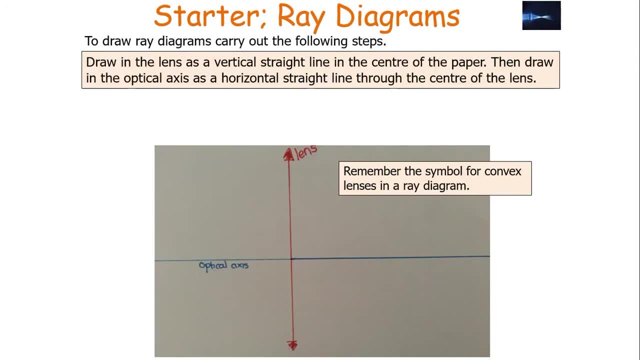 Now this is carried out by drawing a ray diagram for a lens. So to draw a ray diagram, first you're going to draw in the lens as a vertical straight line in the centre of the paper, Then draw the optical axis as a horizontal straight line through the centre of the lens. 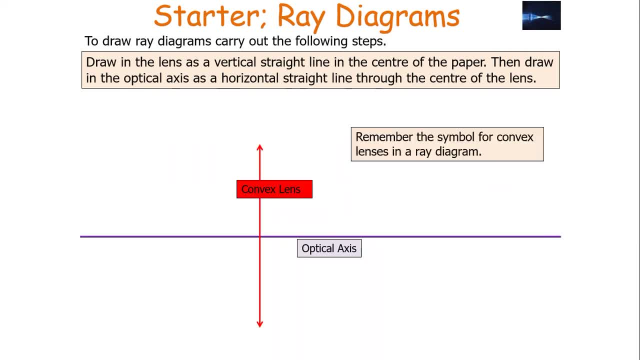 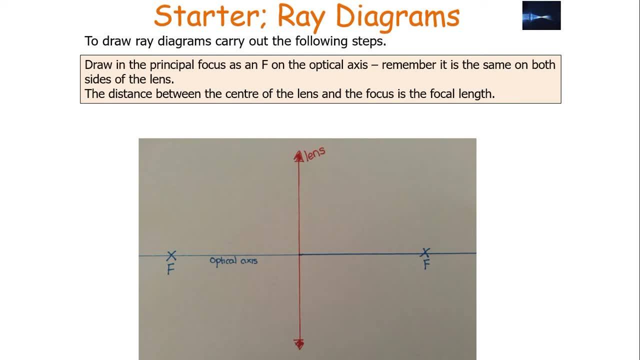 remembering your symbol for convex lenses or convergent lenses in this type of diagram as shown here, Then what you will do is you'll draw in your principal focus as F on the optical axis- Now, you've got to remember it's symmetrical on either side of the lens, So you'll draw. 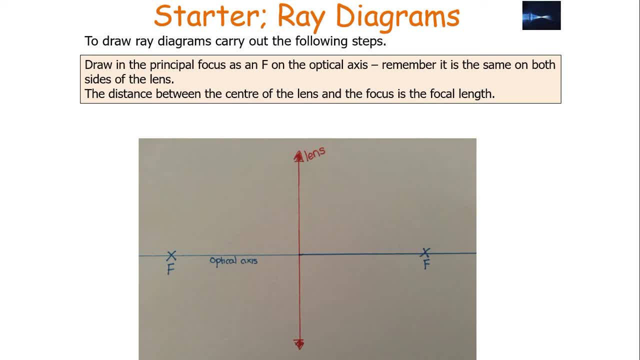 in the focal length. So the distance between the centre of the lens and the focus, or F, is the focal length and it's got to be the same on both sides. So that could be the focal length and that's the focal length and for all lenses it's assumed the focal length is. 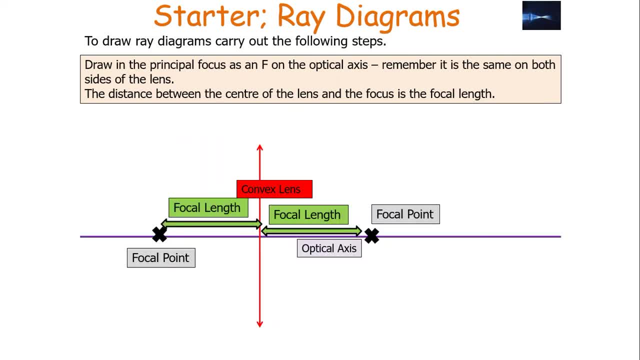 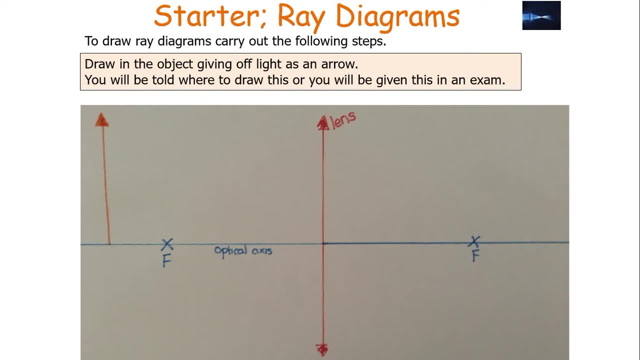 symmetrical on either side of the lens, as shown in this particular diagram. Now. you will then draw in the image given of the radiation, as an arrow It tends to be. you'll be told where to draw this or you'll be given it in the examination. Now the top. 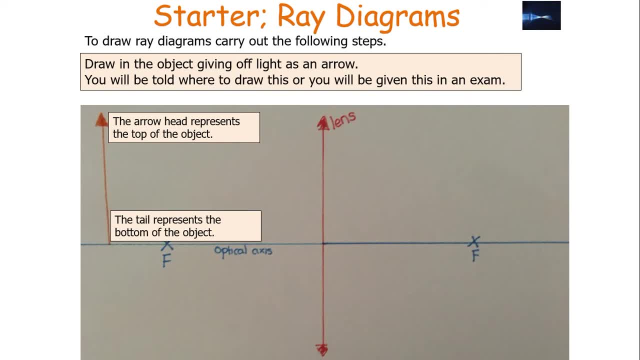 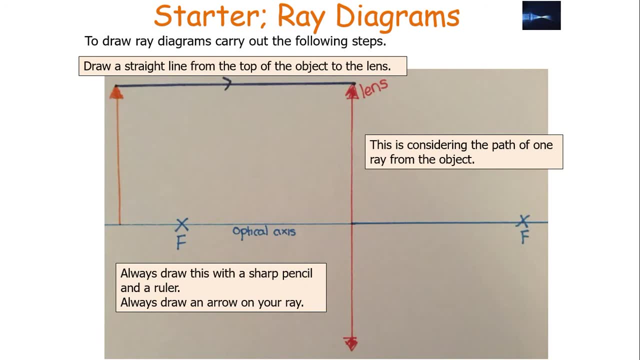 of the arrowhead represents the top of the object. The bottom of the arrow, or the tail of the arrow, represents the bottom of the object as shown here Now, as indicated in this particular diagram. Now, the first thing you would do is you draw a straight line from the top of the object to the lens. So we're considering: 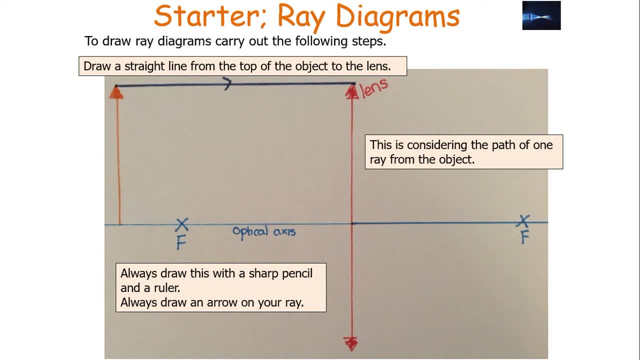 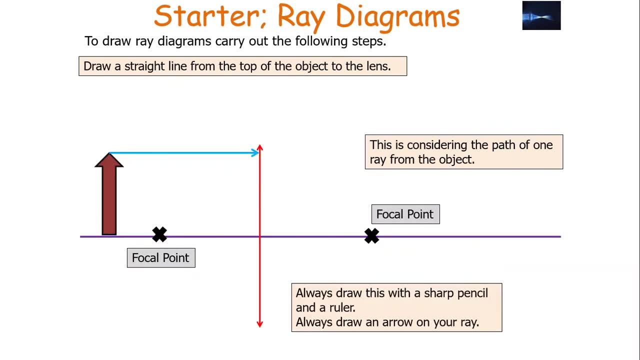 just the path of one ray being emitted from the object. Now, you always draw this with a sharp pencil and a ruler, and you always draw an arrow on your ray, as shown here Now. the rule is that this line will then go past the focus. 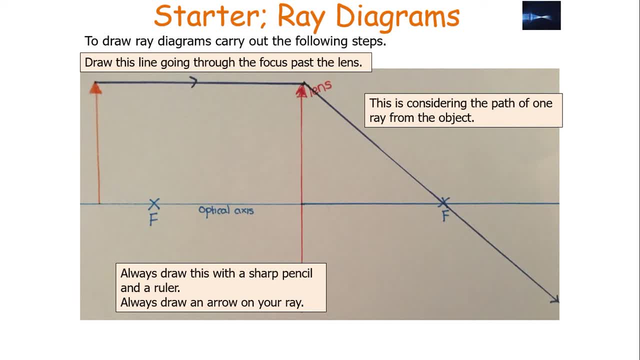 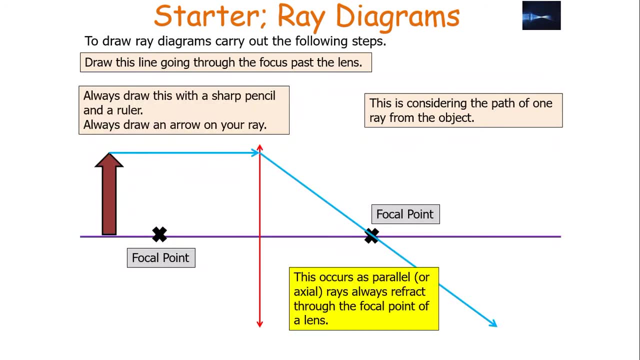 So through the focus, after it goes past the lens, it will refract through the focal point or the principal focus. Now, that's a very important factor to remember in that situation and it comes from our previous definition, because we said that all axial rays will refract. 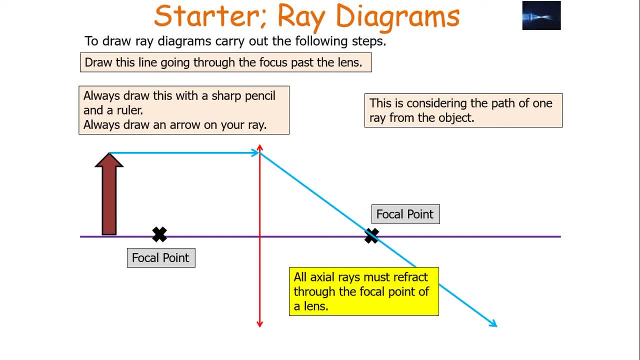 through the focal point of a lens, by definition. So all axial rays, which this ray is, because it is parallel with the optical axis, that purple line, they must refract through the focal point of a lens. So that's a very important idea. 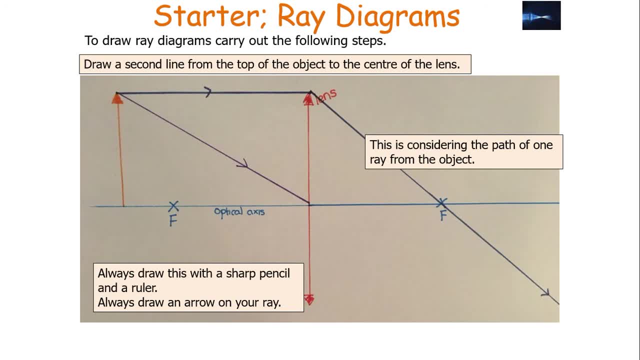 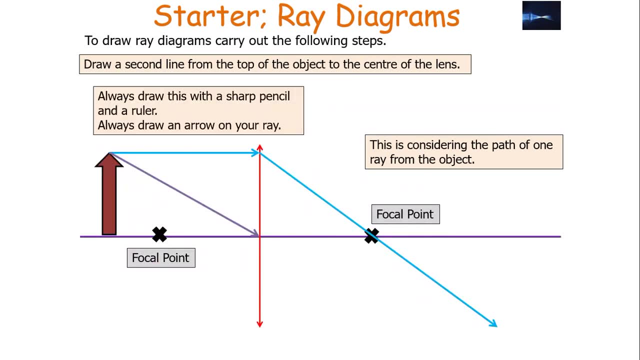 It comes from the actual definition of a focal point. Now, you will then draw a second line, and this second line will also be drawn with a pencil and an arrow will be drawn on your ray, And this is going to go through the center of the lens. Now, like we mentioned before, 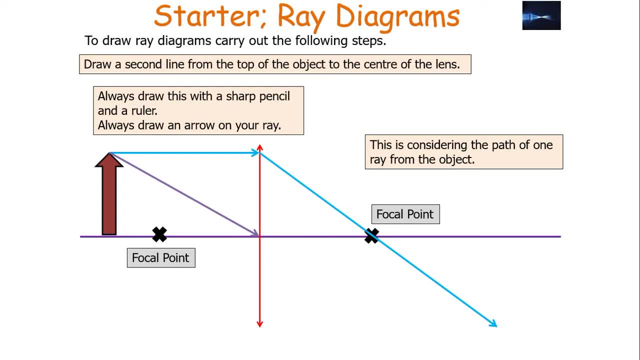 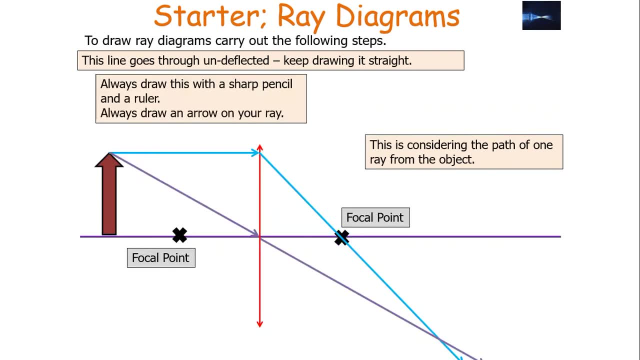 a line going through the center of the lens will go through undeflected. So you continue the path on undeflected, keeping it going in that straight line as shown on this particular diagram. Now, this occurs because there's rays traveling. lens will never refract, they'll just carry through undeflected. now, when the two lines meet, that's. 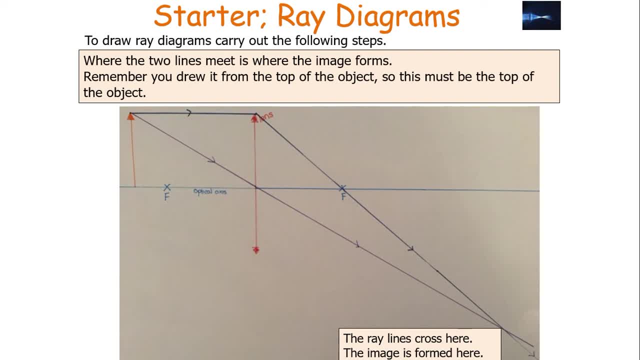 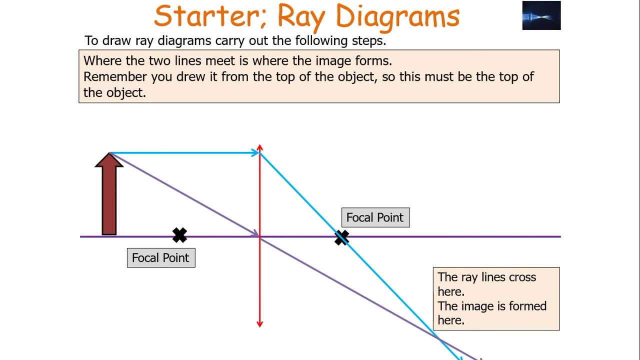 where the image forms. now, remember, you drew it from the top of the object so that that this must be the top of the object. so the rays cross here, so the image is formed here, as shown in the diagram. now it's important to note that it's the top of the object. now, when doing this, you've got to. 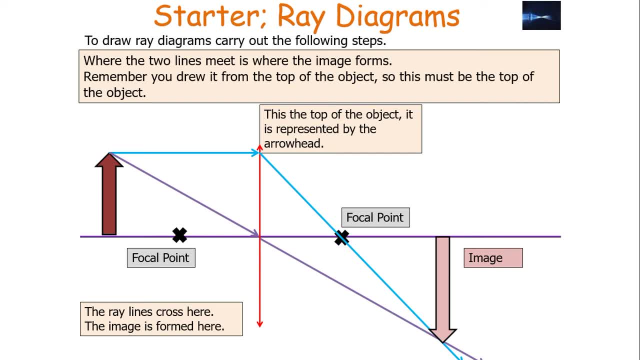 represent this with the arrowhead. so the top of the object is drawn with the arrowhead at the bottom. now this indicates that this particular object is going to be inverted. so this is a real, inverted and magnified image. now it's real because the lines actually cross. it's inverted. 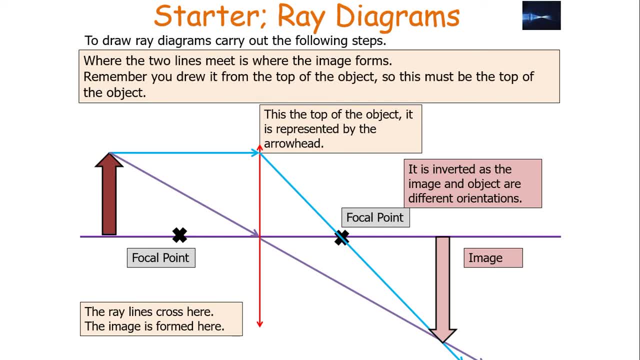 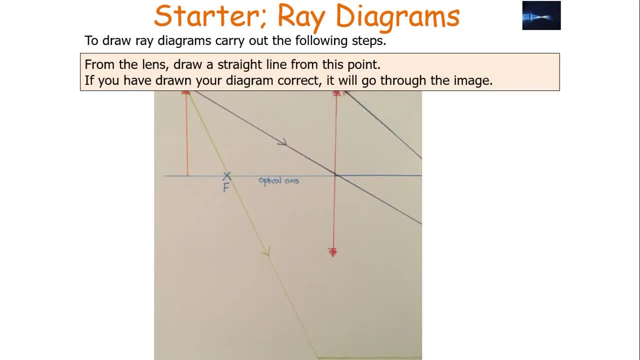 because the image and the object are different orientations from each other. one is facing upwards and one is facing downwards, and it's magnified because the image is larger than the object. now you can also carry out and draw a third line, if you wish so, for this one. 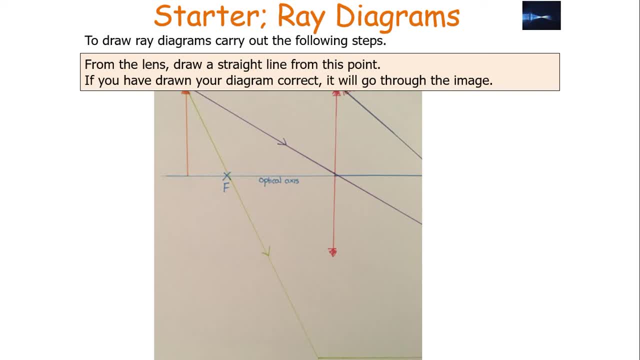 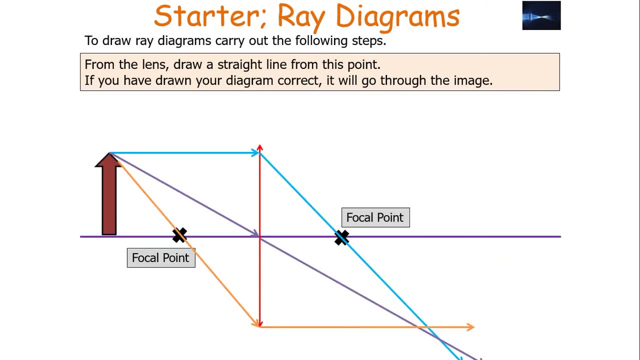 we're going to draw a third line, and we're going to draw a third line and we're going to draw a straight line from the lens. draw a straight line through the focal point on the left hand side of the lens, and what happens is is that when it hits the lens, it will go as a straight line along. 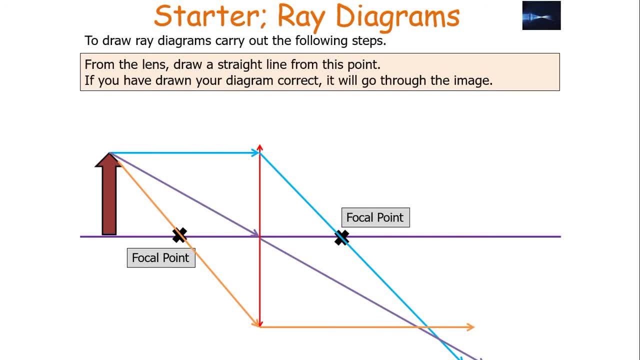 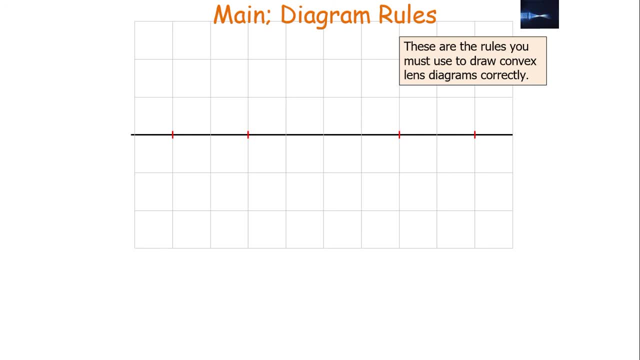 and, as such, it should clarify the and verify that you've drawn your image in the correct place. so let's just clarify what the rules are for drawing in a lens diagram number one. obviously you will draw in your lens and your focal lens and, if you wanted to, two times. 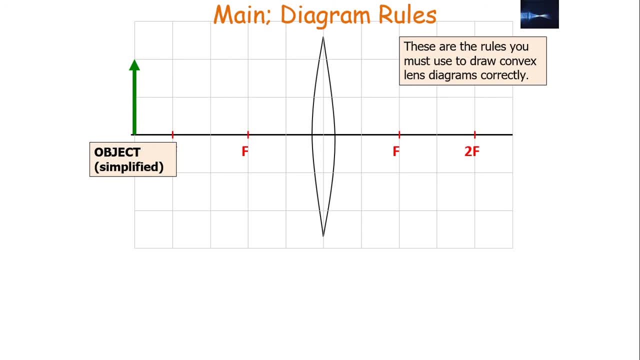 the focal length and if you wanted to two times the focal length and if you wanted to two times the focal length, if you feel it necessary, you will draw a simplified version of your object in. then you will draw a ray parallel to the axis from the top of the object and that line is then. 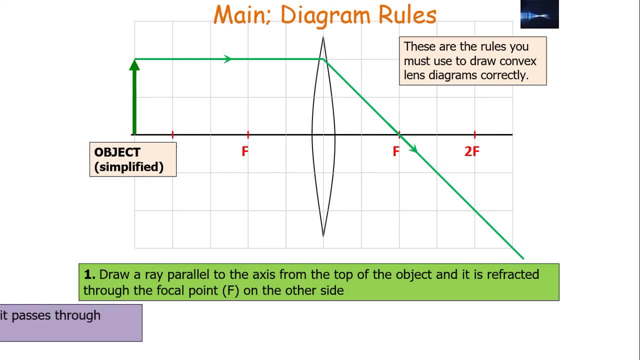 refracted through the focal point on the other side, as shown here. you will then draw in a second ray to the center of the lens from the top and it passes through undeflected. then where the lines cross, that is where the top of the object forms the image forms. i should say. now we can use the 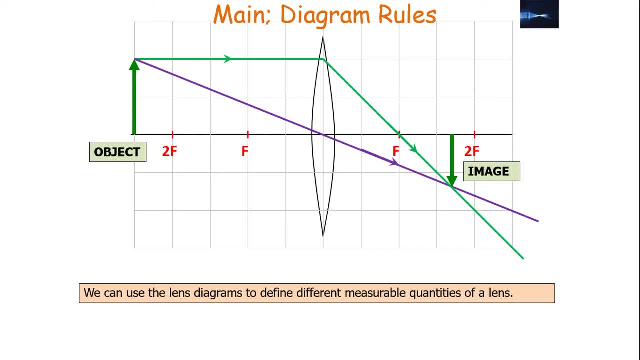 lens diagram to define different measurements of the image and the focal length. if you feel it is a little bit too long, you can also use the lens diagram to define the focal length and the focal length. this will allow us to later derive properties of the telescopes which use these lens. so the first 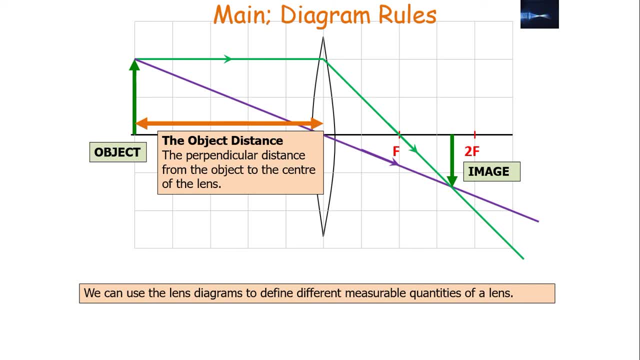 thing we're going to define is something called the object distance. now, this is the perpendicular distance from the object to the center of the lens, and we give it the symbol u. whilst this is the image distance, this is the perpendicular distance from the center of the lens to the image. 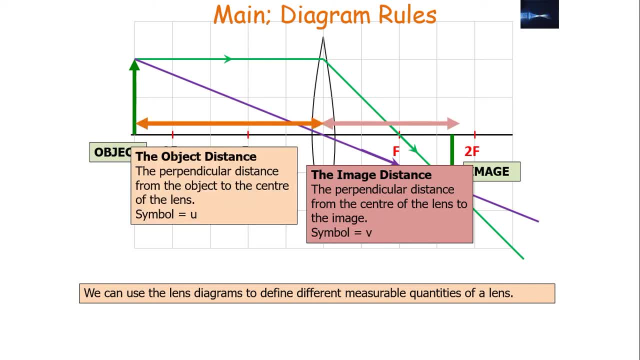 given the symbol v. so we've got our object distance and we've got our image distance, which we can define from our lens diagram we've just provided you with. so we're going to define the current lens intervals using this in the values bar. so the first one we're going to define 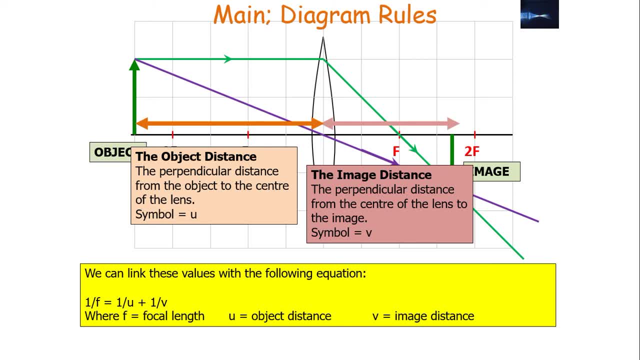 all of the filme values which you just selected are the same paper kanong one, and that is where we define what we're going to be saw: point width, length, distance, right around crime, all of the synergies between the point ratio. okay, here in some of the見 and in some other cubes. 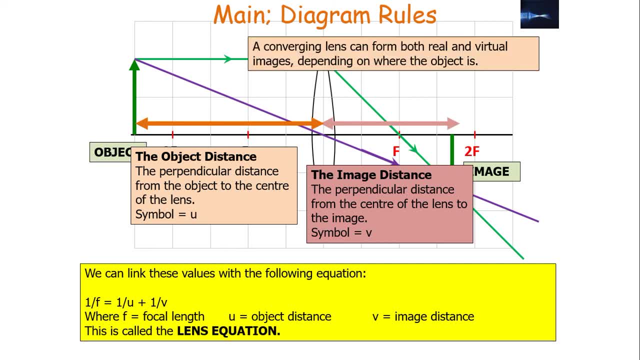 one over focal length is equal to one over. now. that's exactly right and you can. thats exactly how you draw both real and virtual images, depending on where the object is. Now, if the object is further away than the focal length on the image, it'll be real and inverted. but if it's closer than the focal 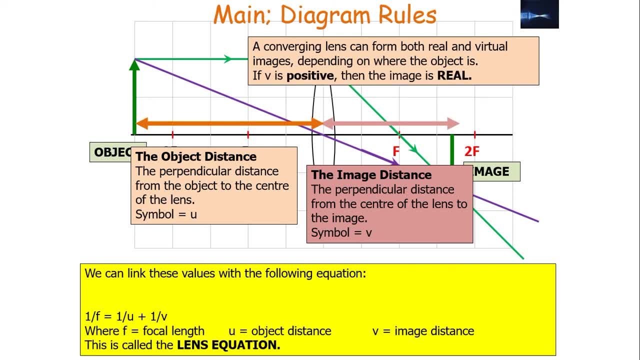 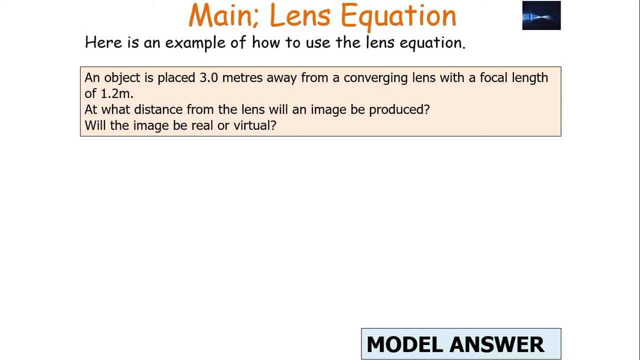 length, the image will be virtual. So if v is positive in this equation, the image is real, but if v is negative, the image is virtual, and that's a very important idea. So we can use this lens equation to work out image distances, but also we can work out whether that image will be real or. 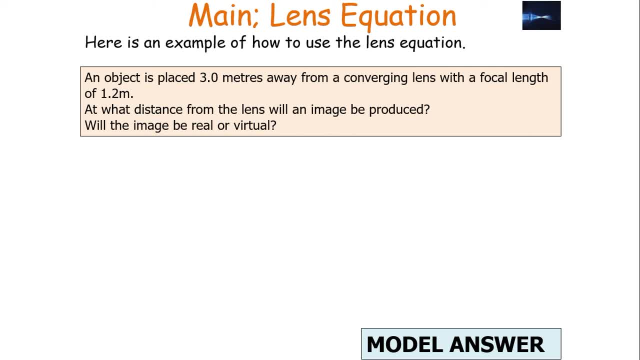 virtual without having to draw the diagram. So let's look at an example question. An object is placed three meters away from a converging lens with a focal length of 1.2 meters. At what distance from the lens will the image be produced? Will it be real or virtual? Well, step one, draw out your 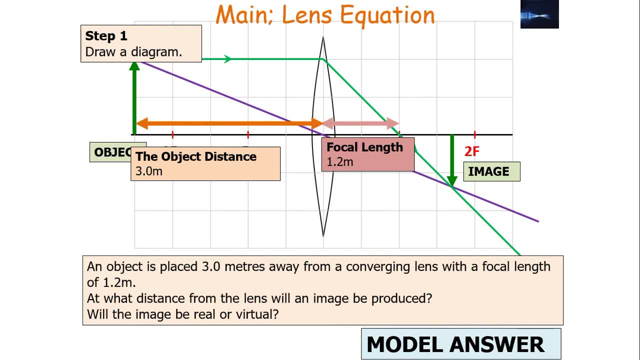 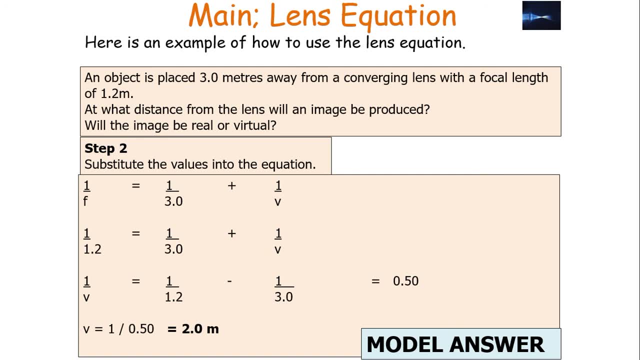 diagram. So we've drawn out our diagram of what's going on in this situation. Step two: draw out your diagram of what's going on in this situation. Step two: we will then substitute the values into the lens equation, So 1 over f equals 1 over 3. 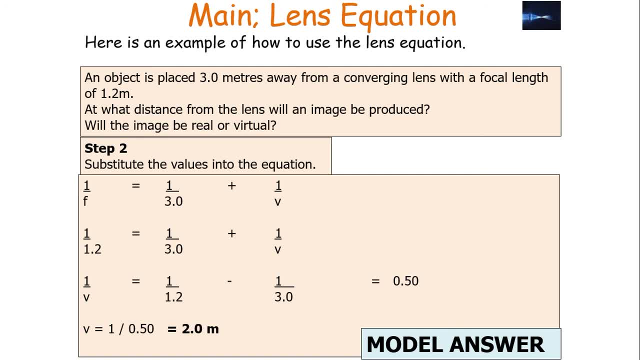 plus 1 over v. So it's 1 over 1.2 equals 1 over 3.0, plus 1 over v. because we've taken those values from the actual equation, We now rearrange it to make 1 over v the subject. So 1 over v equals 1. 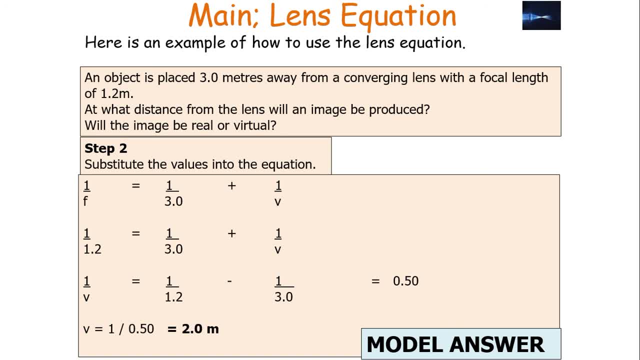 over 1.2 minus 1 over 3.. So the answer is 0.50.. But that's 1 over v. So we've then got to reverse it around. Say v is 1 over 0.50.. So v equals 2.0.. 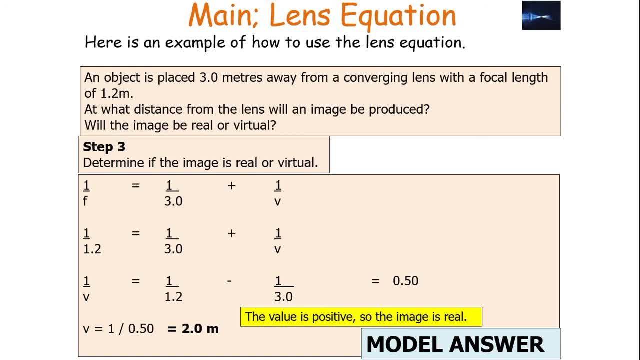 Then, finally, we can use this to determine if the image is real or virtual. Well, this value is positive. It's plus 2.0.. So the image is real. So remember, if the value you work out for v in this equation is positive, the image is real, because this tells us the object is further than the focal. 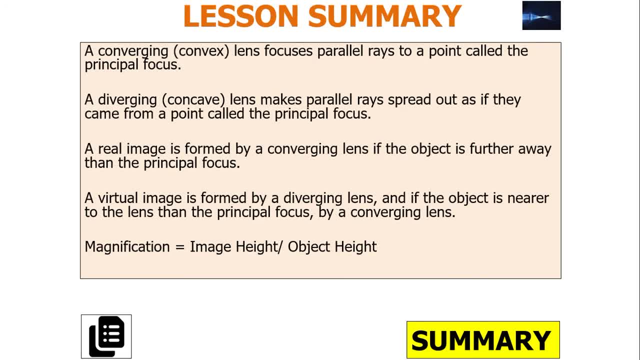 length away from the lens So we can use this to determine if the image is real or virtual. So it has to be real. So what have we learned in today's lesson? A converging or convex lens focuses parallel rays to a point called the principal focus. A diverging lens makes parallel. 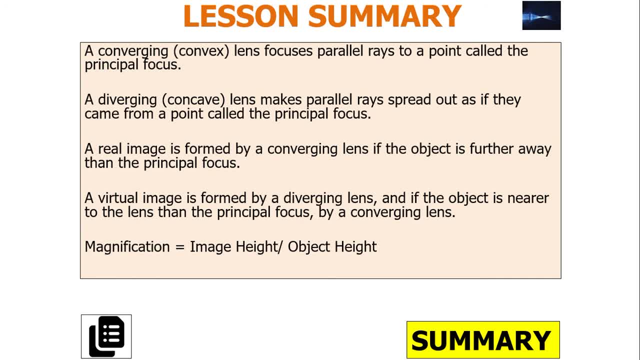 rays spread out as if they came from a point called the principal focus. A real image is formed by a converging lens if the object is further away than the principal focus, And a virtual image is formed by a diverging lens and if the object is nearer to the lens than the principal focus. 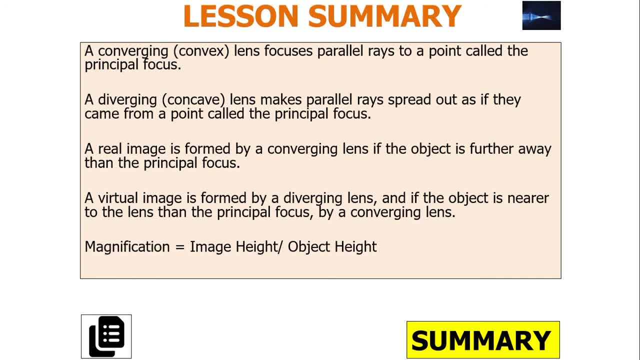 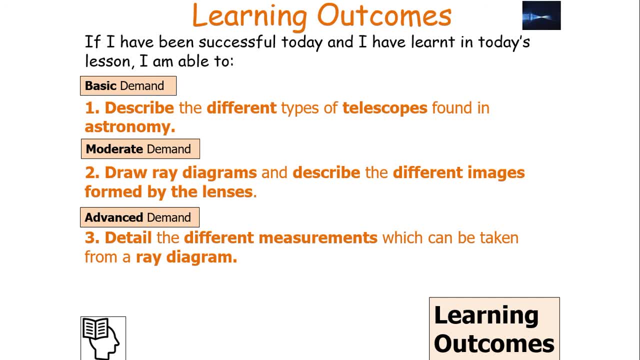 by a converging lens In magnifications. we can use this to determine if the image is real or virtual. So if we've been successful and we've learned in today's lesson, you should be able to describe the different types of telescopes found. 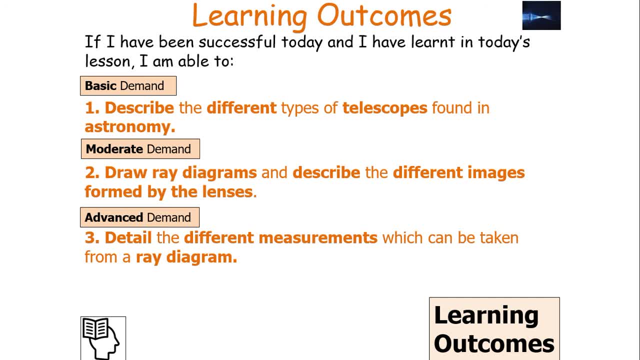 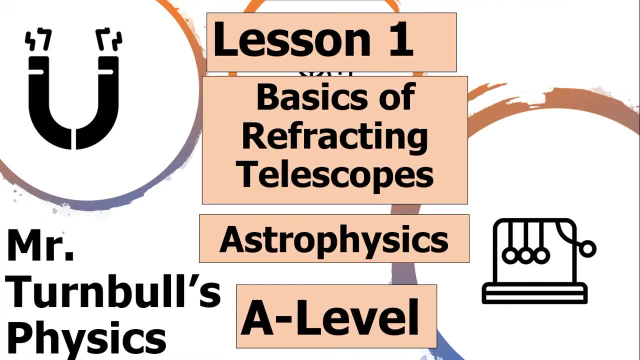 in astronomy, draw ray diagrams and describe the different images formed by lenses and detail the different measurements which can be taken from a ray diagram. I hope you've enjoyed this particular lesson looking at the basics of refracting telescopes and have a lovely day.